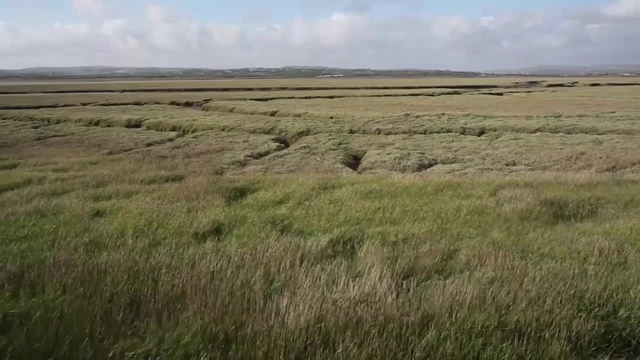 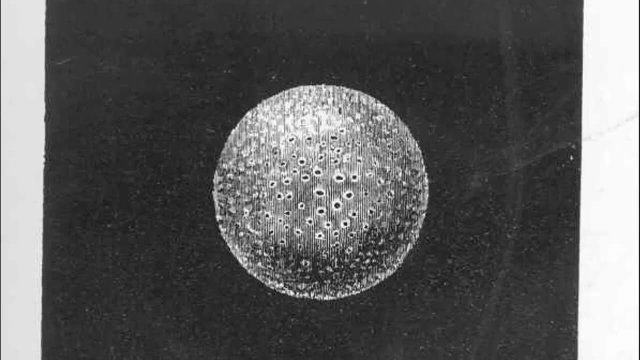 Others are abundant in the deep ocean or on coral reefs. Others are abundant in the deep ocean or on coral reefs. Others only live in brackish estuaries or intertidal salt marshes. The majority of species have shells called tests. The simplest forms are open tubes or hollow. 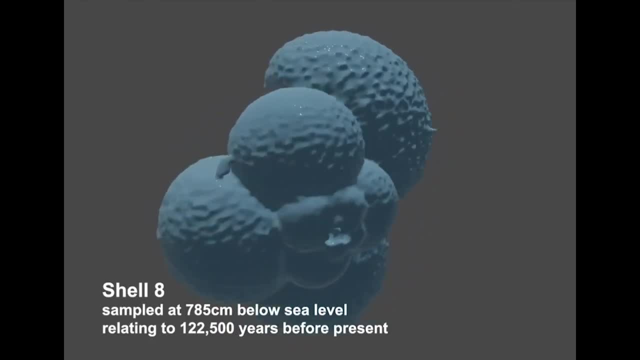 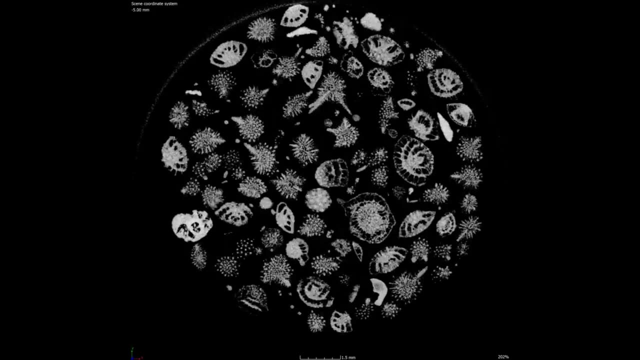 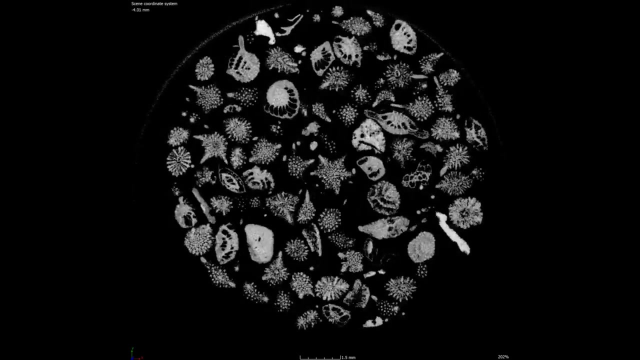 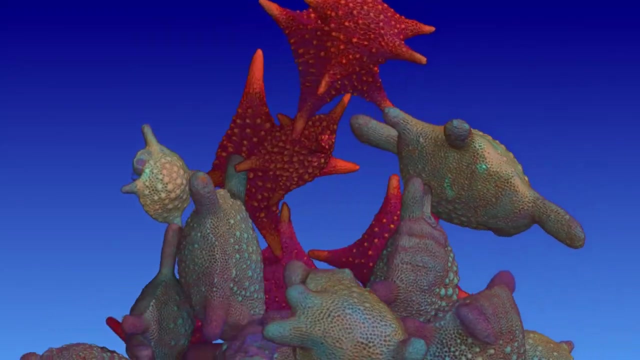 spheres More complex. shells are commonly divided into chambers that are added during growth. The shell may be made of many different materials, such as organic compounds, sand, grains and other particles cemented together or crystalline calcite. The shell may have a smooth or rough surface. Fully grown individuals range in size from about 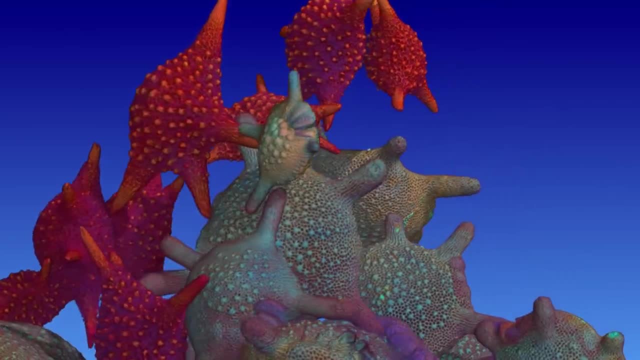 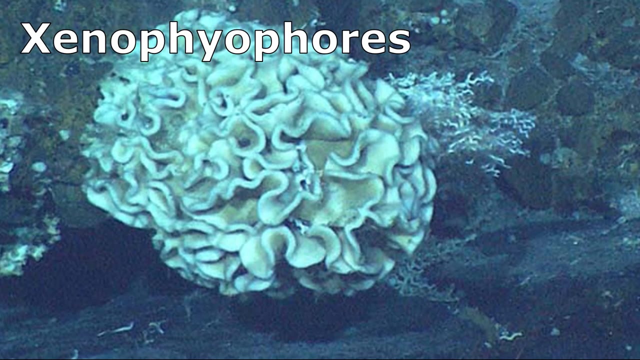 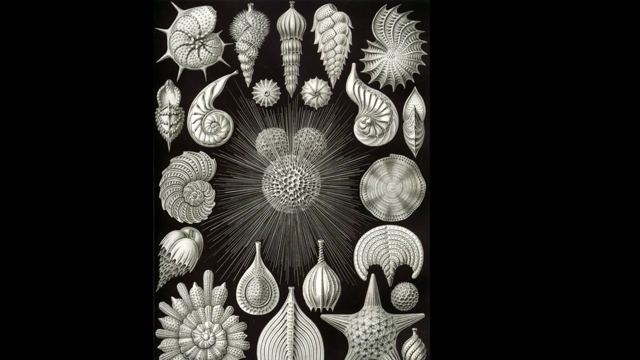 100 micrometers to almost 8 inches long. One group, the Xenophyophores, can grow to several inches in size as a single cell. A single form may have one or many nuclei within its cell. Forms eat foods such as dissolved organic molecules, bacteria, copepods and other. 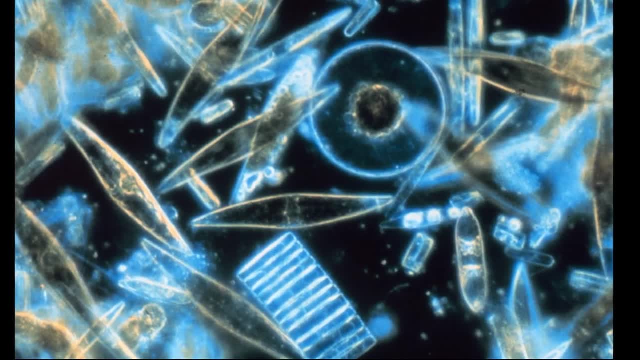 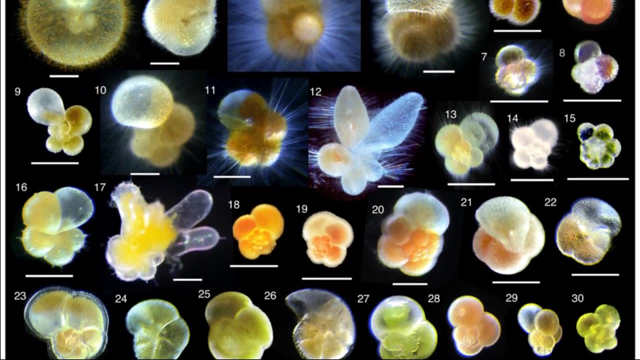 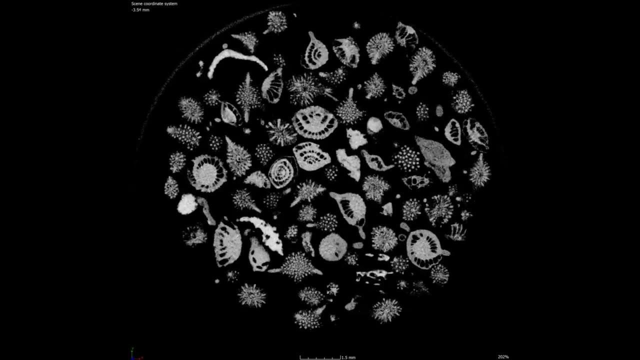 compounds and single-celled phytoplankton like diatoms. Some species that live near the surface have a symbiotic relationship with unicellular algae that they farm inside their shells for food. Others that live in low-oxygen environments form symbiotic relationships with chemo-autotrophic 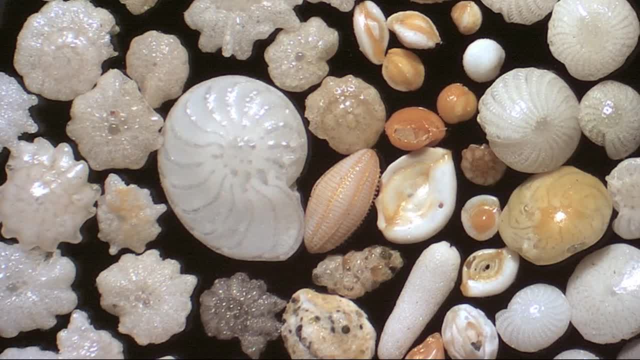 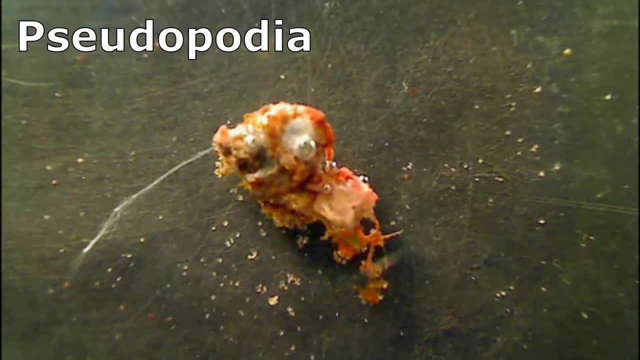 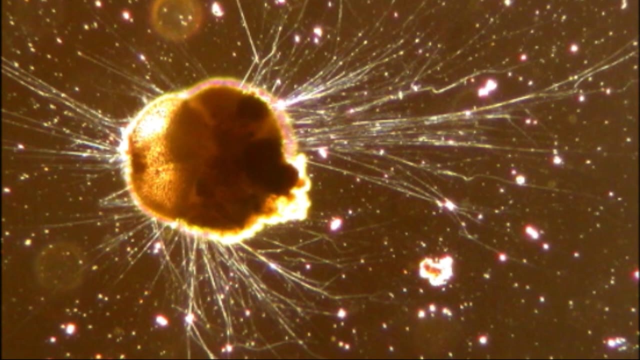 bacteria. Some species are parasitic Forms can move and catch their food with a network of pseudopodia that are thread-like extensions of the ectoplasm. Under the microscope these pseudopodia appear granular. The pseudopodia are called reticulopodia. They extend from one or more holes in the shell. 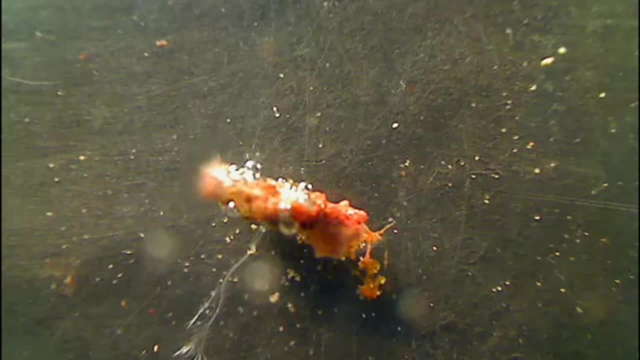 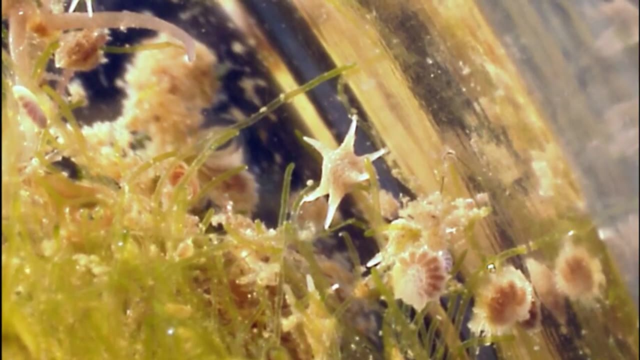 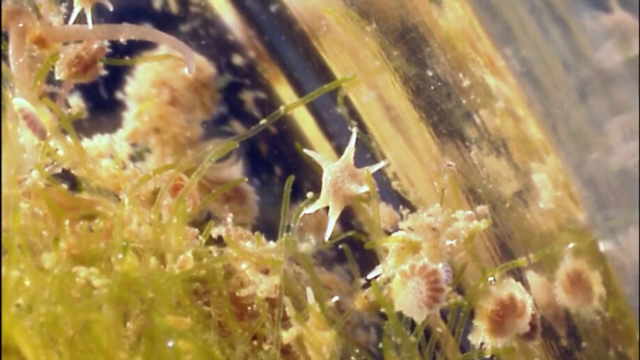 The pseudopodia transfer material to the inner shell and back. They can be extended and retracted. Bottom-dwelling foraminifera may also use their pseudopodia for locomotion and anchoring. Some benthic species slowly burrow through sediments at speeds of up to a half inch per hour. 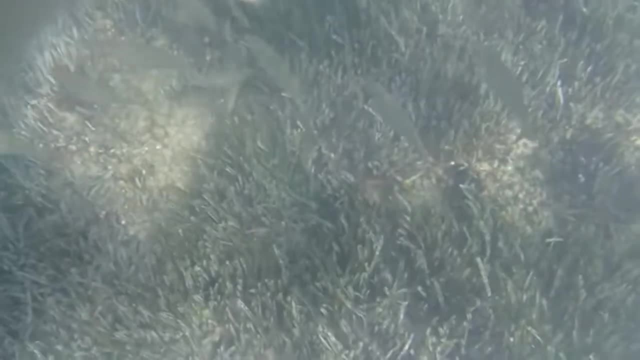 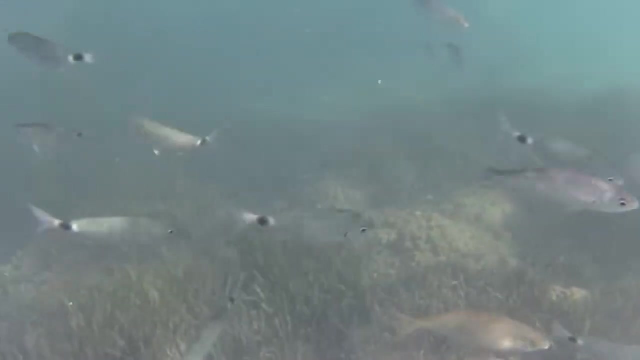 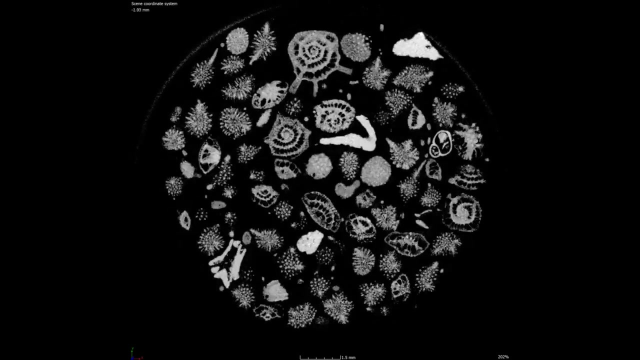 Others attach themselves to the surface of rocks or marine plants. Bottom-dwelling forams play a significant role in the benthic carbon and nitrogen cycles. Forams have many predators, such as worms, crustaceans, gastropods, echinoderms and fish.